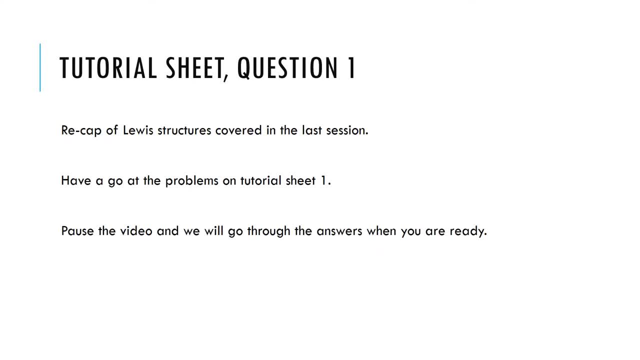 using VSEPR theory. So in the relevant section on Moodle you will find a tutorial sheet. I would like you to have a go at question one on this tutorial sheet. This recaps some of the stuff we were talking about last time with regards to Lewis structures and, of course, 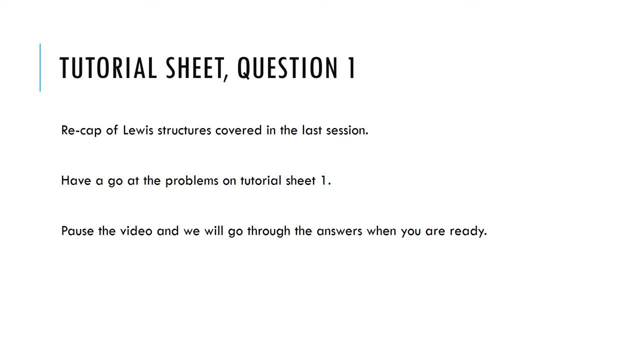 Lewis structures are really important because they're the first step in predicting the shape of a molecule through VSEPR theory. So I suggest that you pause the video here. have a go at question one on tutorial sheet one and we will go through the answers when you are ready. 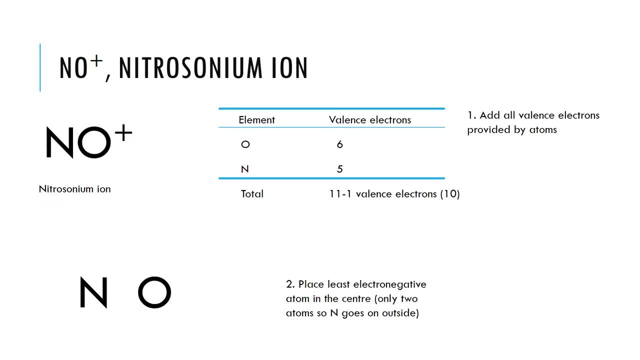 Okay. so question 1a will ask you to write the Lewis structure for the nitrosonium ion NO plus. Well, the first thing we've got to do is add all of those valence electrons which are provided by the atoms. So oxygen has six valence electrons and nitrogen has five valence electrons. That 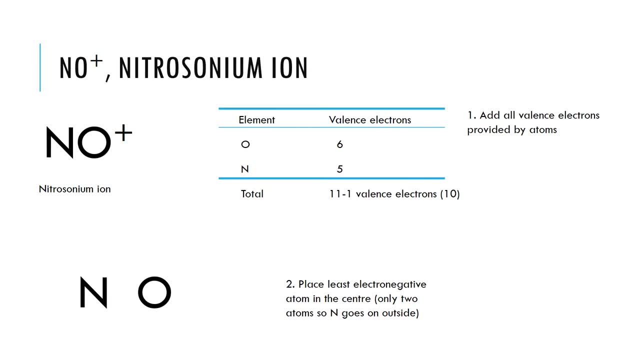 gives us a total of eleven valence electrons. So that gives us a total of eleven valence electrons. but remember, now we have to subtract one, because there's a positive charge associated with this nitrosonium ion. There's an electron missing there somewhere, So we subtract one from the count and 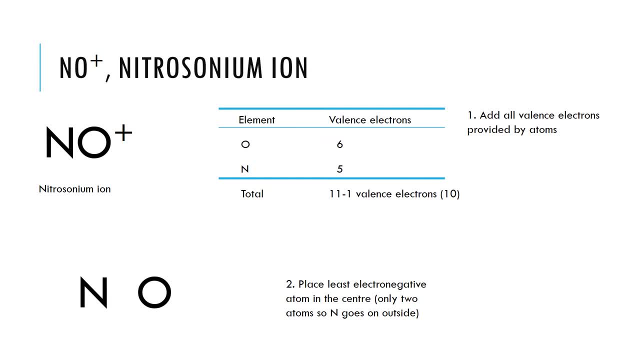 we obtain ten valence electrons. Step two in the construction of a Lewis structure is to place the least electronegative atom in the centre. Well, there are only two here, so we'll stick nitrogen on the outside. We then place two electrons between the atoms to form a chemical bond and we complete the octets on the outside atoms. 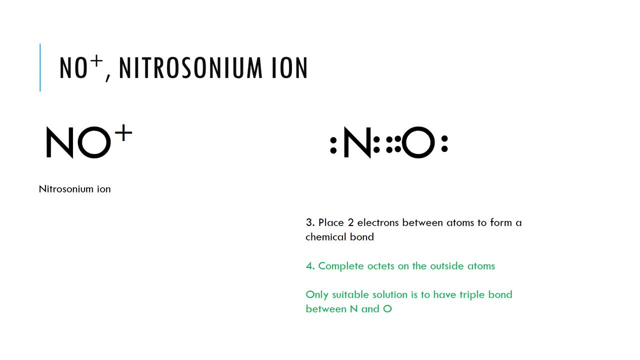 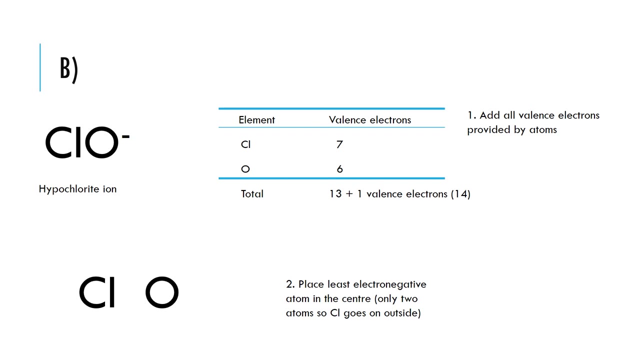 And you'll note here that the only suitable solution to the Lewis structure, the only way to gain a complete octet for all atoms in that molecule, is to have a triple bond between nitrogen and oxygen, The hypochlorite ion, then CLO minus. Again we add all of those valence electrons. 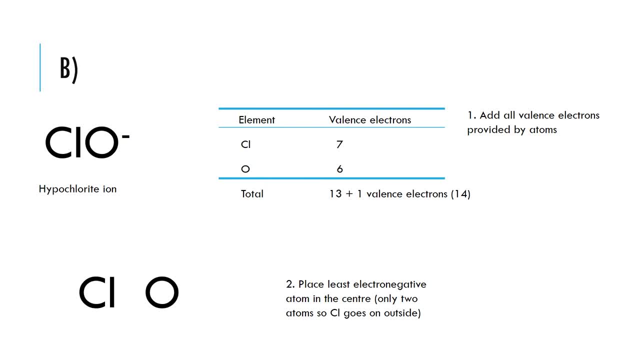 And we obtain a total of 13 valence electrons. but remember, there's a negative charge associated with this molecule, So we've got to add an electron because there's an extra electron in this system. We place the least electronegative atom in the centre. Well, again, there are only two. 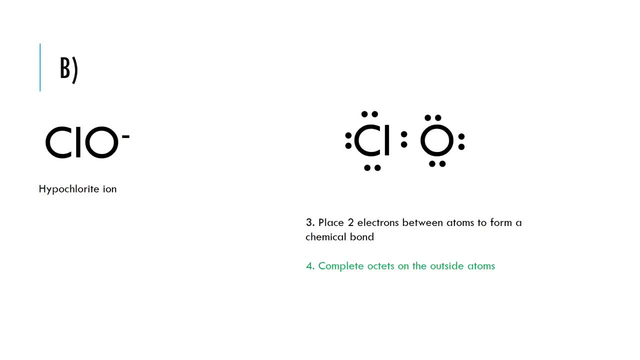 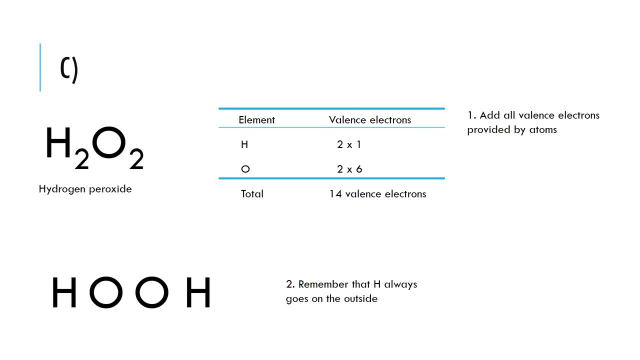 So we'll put chlorine on the outside. here We place two electrons between the two atoms to form a chemical bond, And if we complete the octet on all of those atoms, then the solution is shown there. Question 1C is hydrogen peroxide, H2O2.. 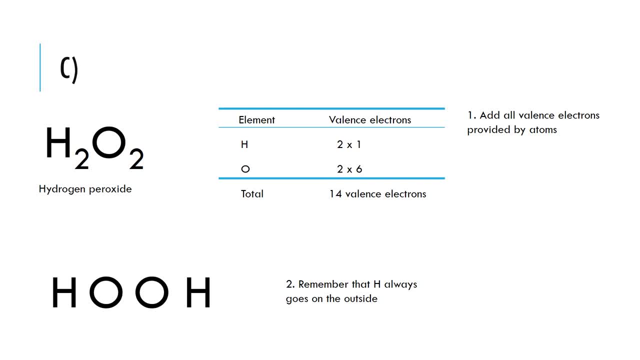 We add all of the valence electrons in the system, That gives us a total of 14 valence electrons. We stick the least electronegative element in the middle? Well, in this case no, because you remember that hydrogen always goes. 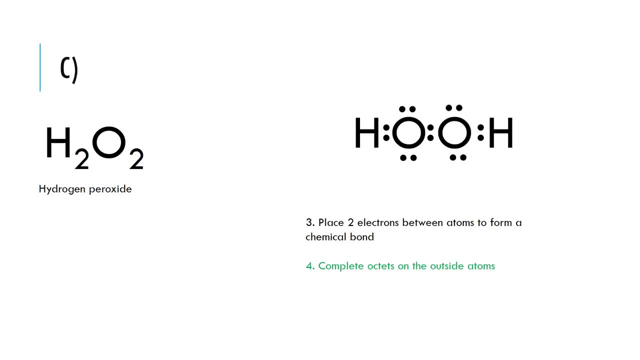 Goes on the outside. So the oxygen sits in the middle. here We place two electrons between the atoms to form a chemical bond, and we complete the octets on those outside atoms. The solution is shown there, Remembering then that hydrogen only needs two electrons to complete its outer shell. 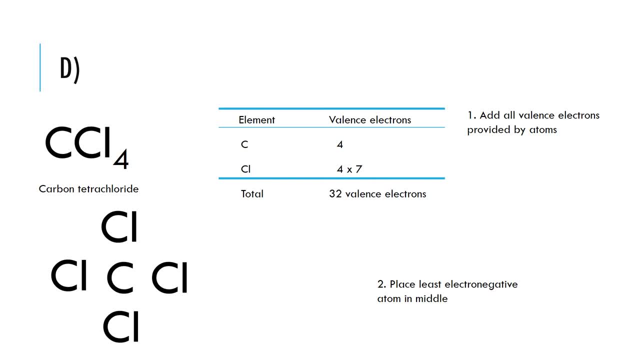 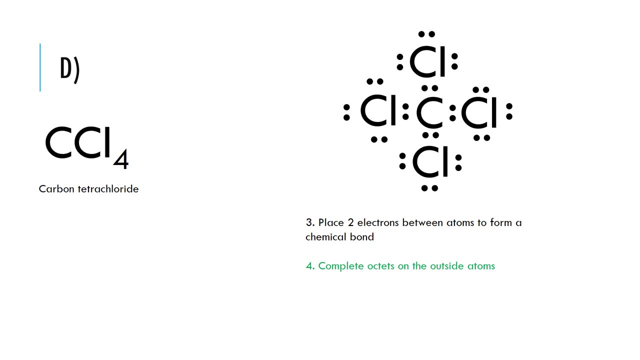 Question 1D is carbon tetrachloride, CCL4.. A total of 32 valence electrons In this system. we place the least electronegative atom in the middle, which is carbon, And we place two electrons between the atoms to form a chemical bond. 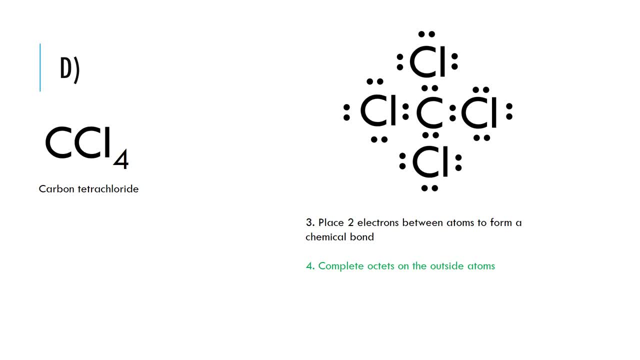 And finally we complete the octets on the outside atoms, And this looks a bit messy. This is a bit of a messy one. Normally we'd probably put just draw a straight line between the carbon and the chlorines here to show a bond, an implicit sharing of two electrons. 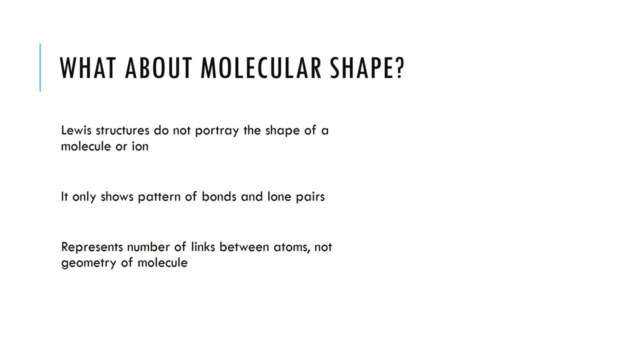 So we said last time then that Lewis structures don't portray the shape of a particular molecule or ion. We're only looking at a pattern of bonds and lone pairs And in fact they only represent the number of links between the atoms, But not the geometry of the molecule. And we said that VSEPR theory is really important. 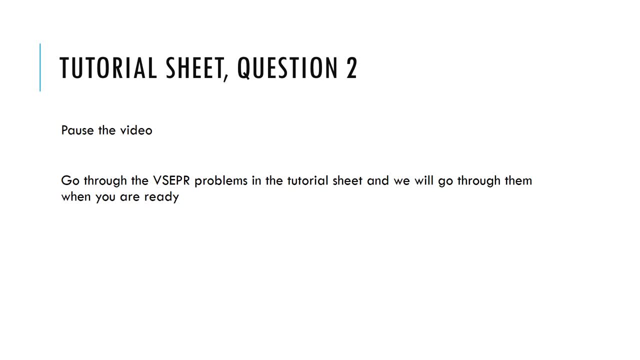 VSEPR theory is really important because we can predict molecular shape Using VSEPR theory. So again, I want to cement some of the concepts that we spoke about last time And For you to have a go at these tutorial questions. 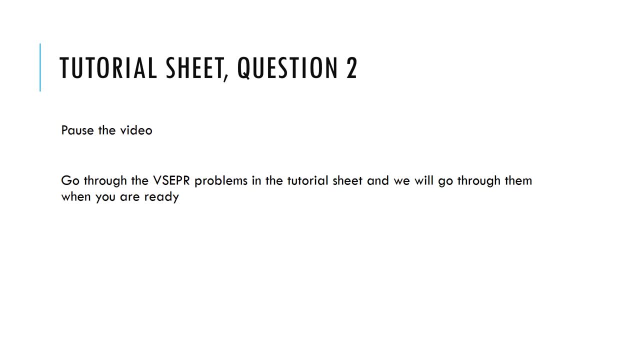 So this is now question two on the tutorial sheet for this week. Have a go at them and we'll go through the answers when you're ready. Just pause the video and I'll go through the answers when you resume. OK, so question one A: Sulphur trioxide. 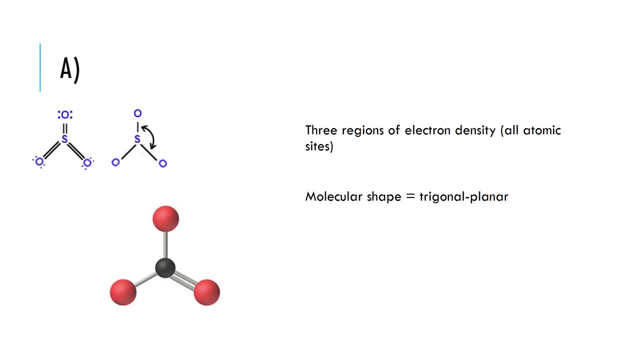 Three regions of electron density here. All of them are atomic sites, So the molecular shape is the same as that basic arrangement that we spoke about last time. It's trigonal planar. Question one B then is now the SO32- There are three atomic bonds here and a lone pair on sulphur. 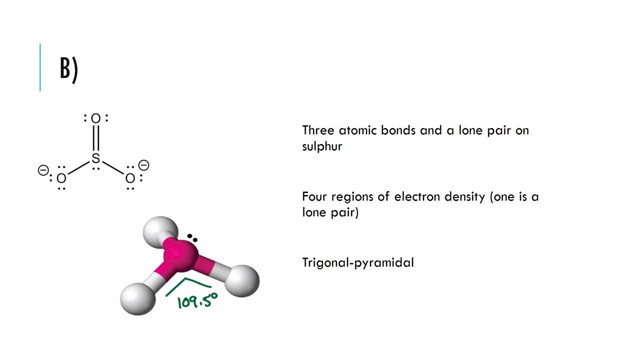 So there are four regions of electron density, But remember one of those is a lone pair, So the shape of the molecule is trigonal, pyramidal. Basic arrangement of the molecule. That's when we described the distribution of regions of enhanced electron density. Is tetrahedral, But only three of those are atomic sites, So the molecular shape is trigonal, pyramidal. One C is a very strange molecule, IF5.. There are six regions of electron density here. Only five of them are atomic sites. 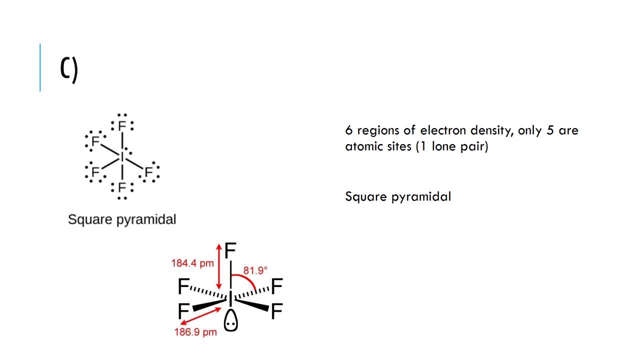 Only five of them are iodine fluorine bonds. One of them is a lone pair, So we described the molecular shape of this molecule as square, pyramidal. One D, then IF6.. Another strange molecule: Six regions of enhanced electron density. 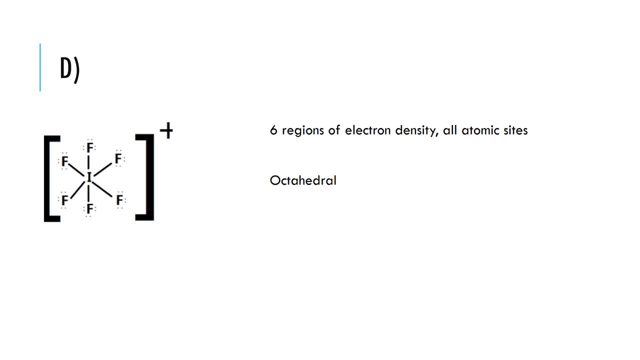 All of them are atomic sites, So we describe the molecular shape of this molecule as octahedral. And finally one E XEF4O- Six regions of enhanced electron density there, But one of them is a lone pair. Only five of them are atomic sites. 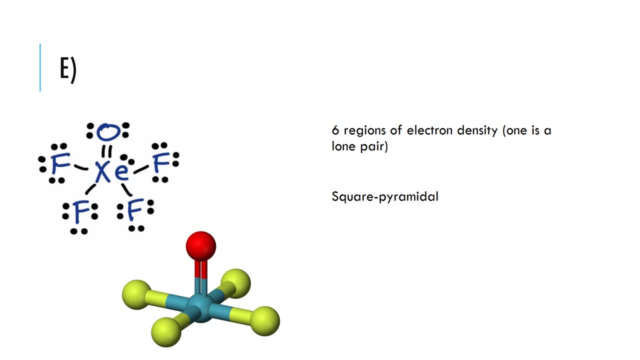 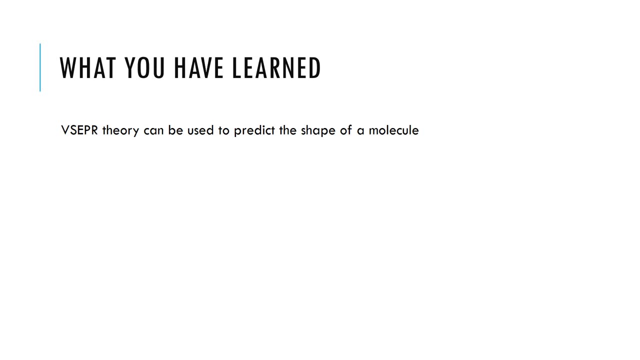 So the shape of the molecule is square, pyramidal, So hopefully you got on OK with those. Please do contact me if there are any issues in going through the tutorial questions. You can contact me via email Or Microsoft Teams. Thank you very much.